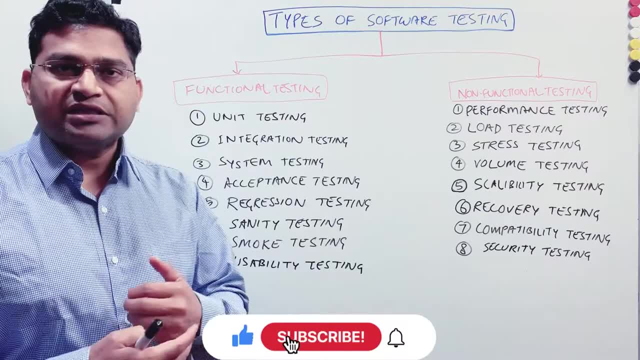 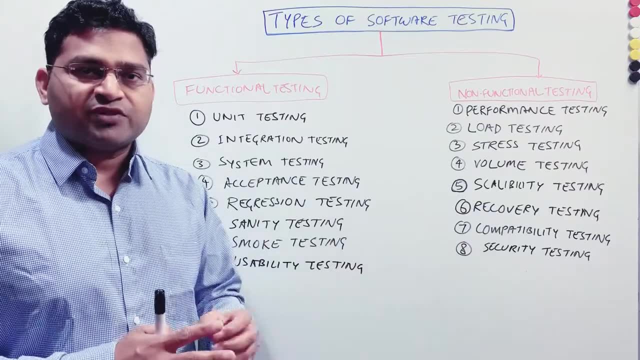 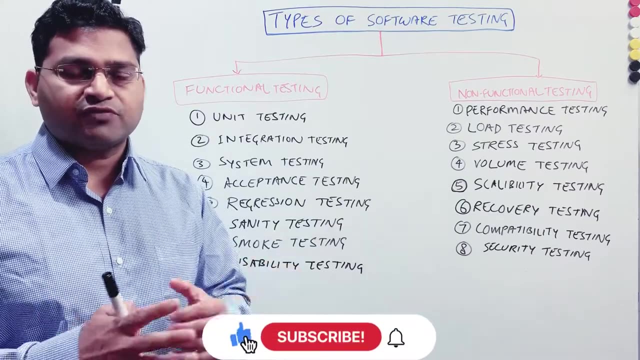 testing. there are so many types of testing, right, So any type of or any testing that you do within the software testing project can be categorized as type of testing, And if you try to browse around and try to search on Google, you'll find hundreds. you know almost hundred. you know types of. 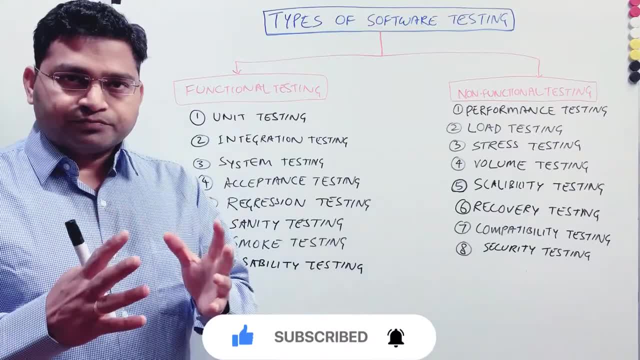 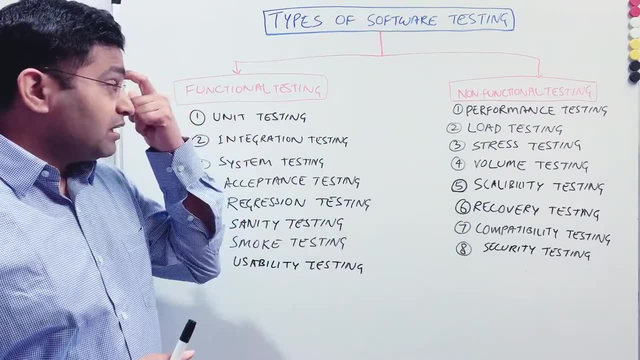 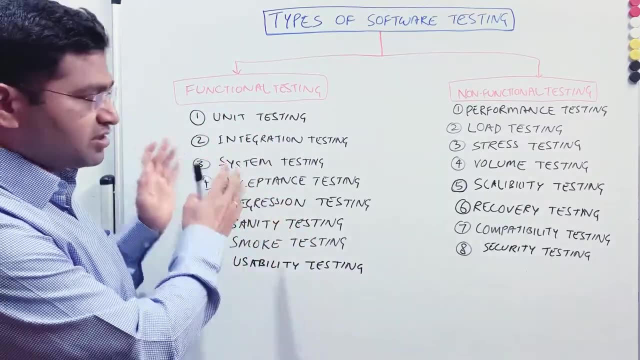 testing, different types of testing. So let us first understand the broader category of the type of testing. So if you see, on my board here I have categorized. So in the broader sense the types of testing can be categorized either into the functional or non-functional category. 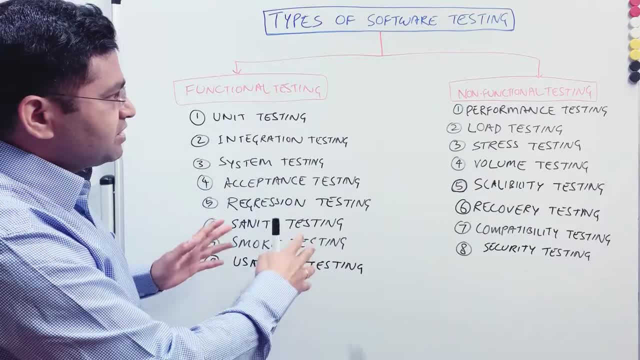 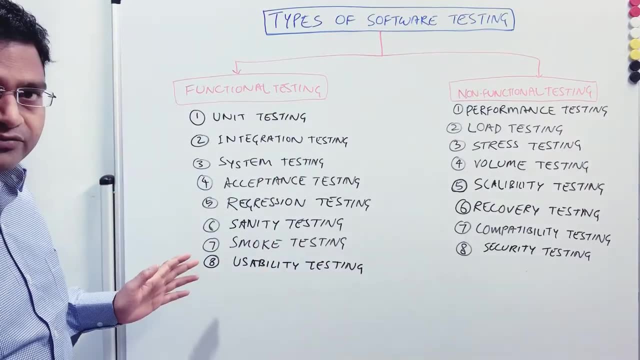 And that is why I have categorized these- you know types of testing- into functional and non-functional category, And in the functional category there are some testing types that I have noted down here And similarly, in the non-functional category, I have noted down. 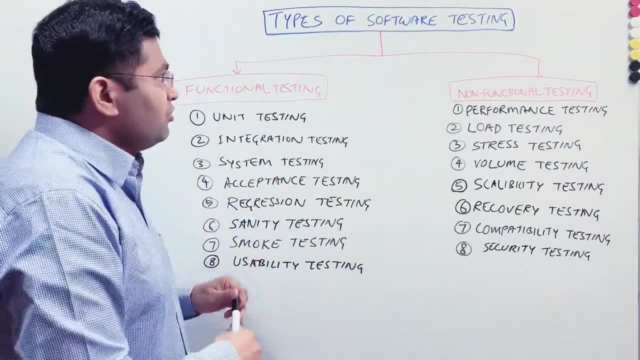 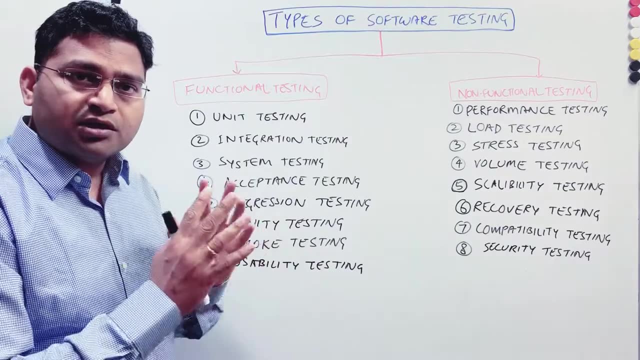 some of the categories, some of those. So let us first understand the broader category of testing. Now, if you talk about the types of testing, so these are not the only type of testing that are available out there. If you go ahead and search Google, you'll find the types of testing And 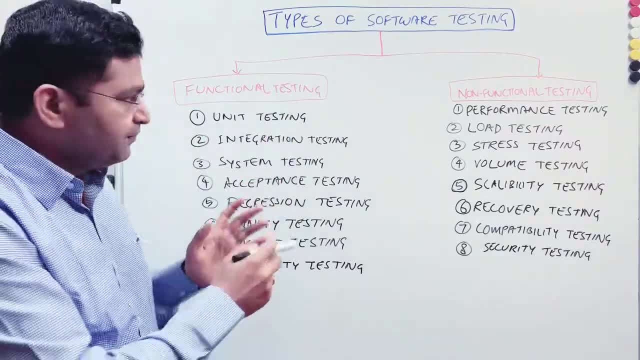 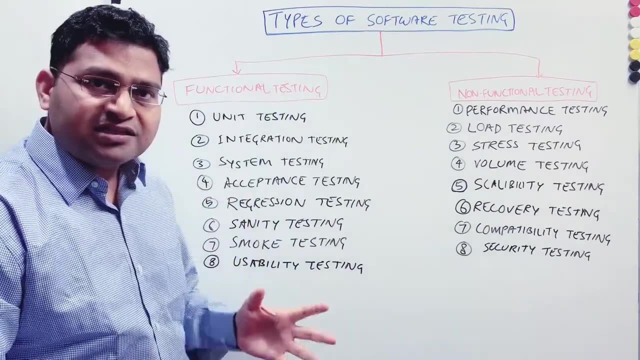 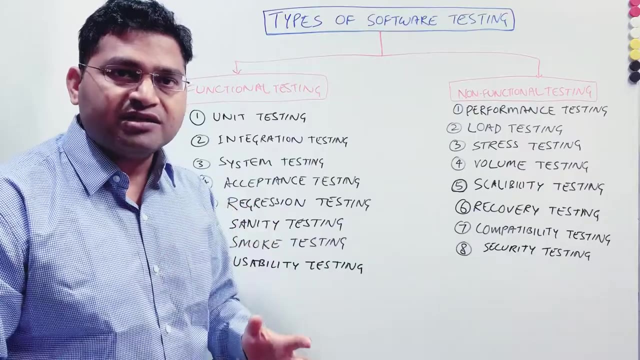 mostly, you can categorize those testing that you will find into either functional or non-functional category, right? So when we talk about the type of testing, it is any testing that you'll perform, okay, And when we say functional testing, it is basically the testing of the functionality. 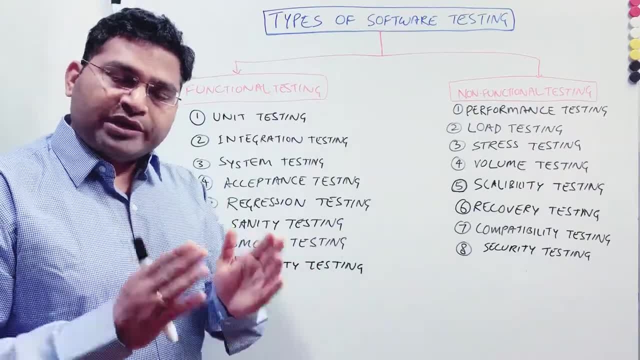 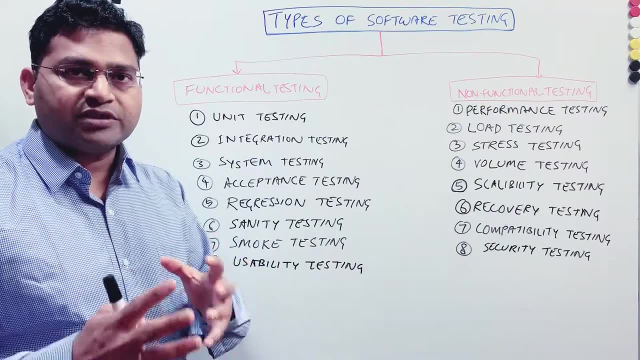 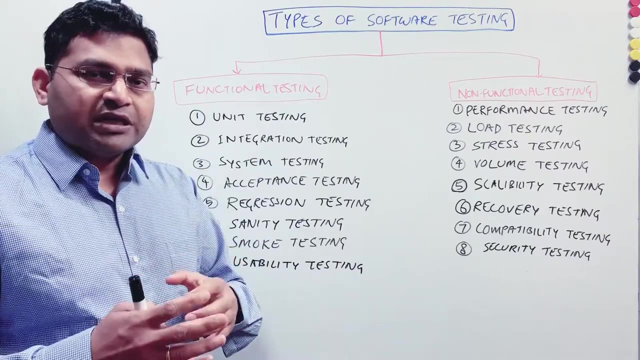 of a particular software right. So whenever a customer provides you the requirement, they will basically provide the functional requirements. So, for example, again taking the e-commerce website customer will provide the requirements. So, for example, I want to have the registration functionality right, So that's the functionality that needs. 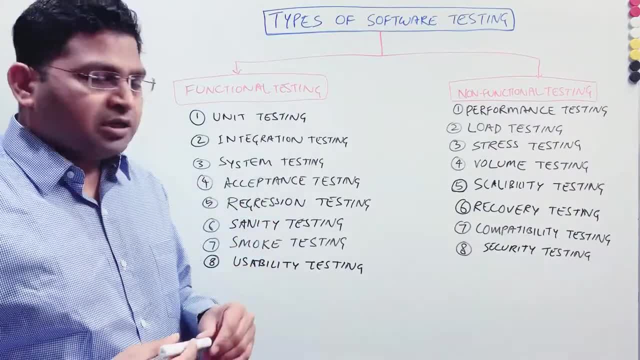 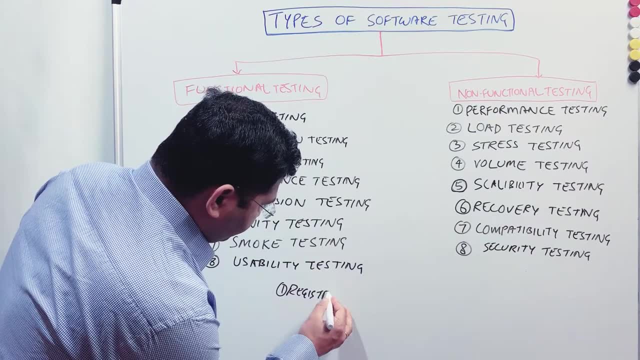 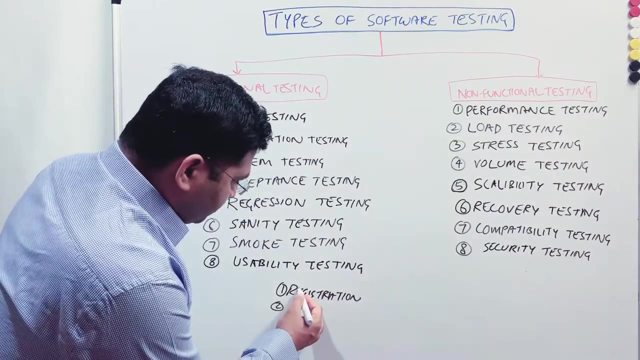 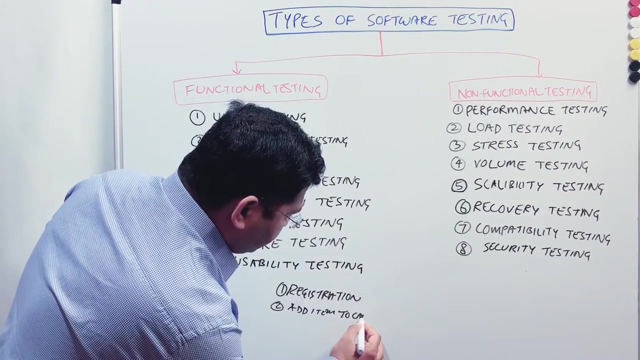 to be built into the e-commerce website. So registration functionality will be one, So registration, So that's one of the functionality, right. And then say, for example: you know, the other functionality is add items right, Add items to cart, right. So these are same. 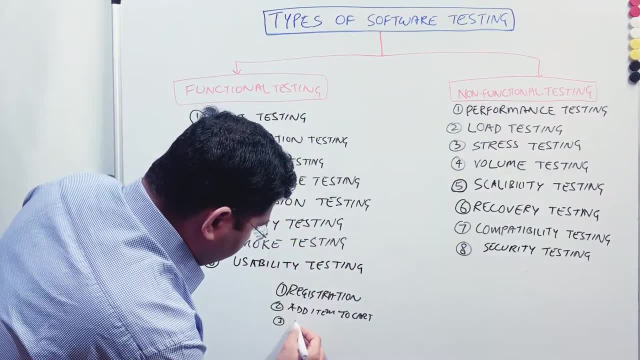 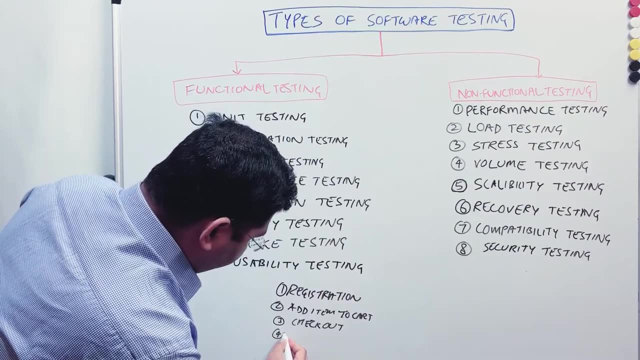 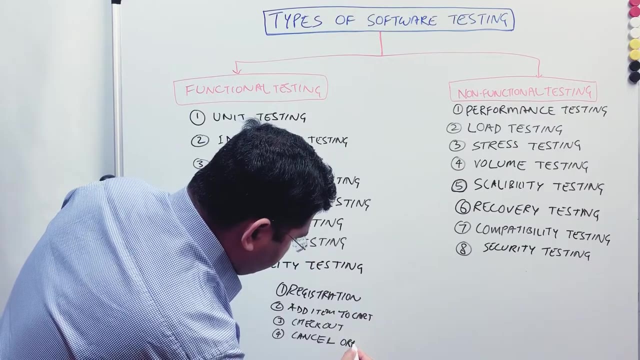 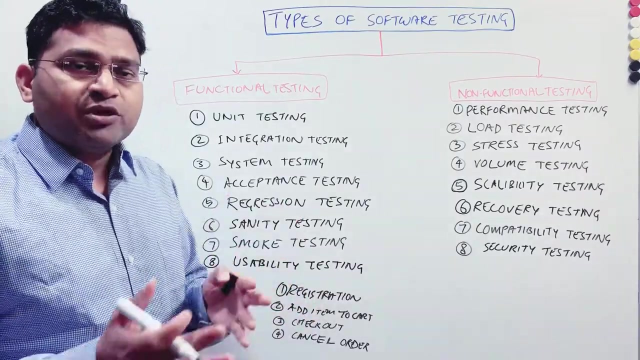 examples that I'm taking from the previous tutorials. Then checkout: all right, So another functionality Or cancel order: User should be having a functionality to cancel the order. okay, So these are some of the functionalities or functional requirement that might be available or might be required for an. 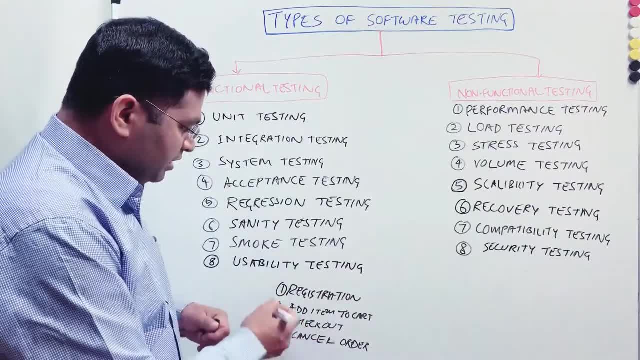 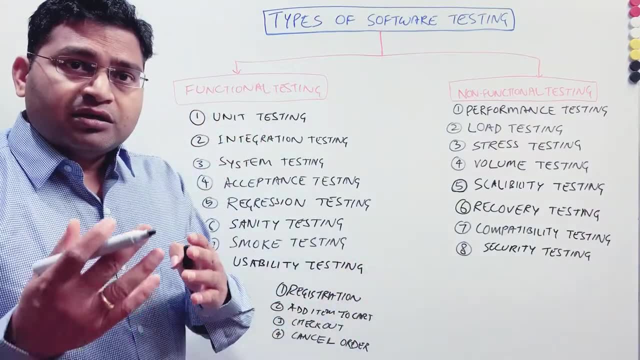 e-commerce website, if a customer wants to build an e-commerce website. Now, when we talk about the non-functional requirement or the non-functional testing, the non-functional testing tests, the non-functional aspects, So, for example, how the performance is. Now, when we talk about 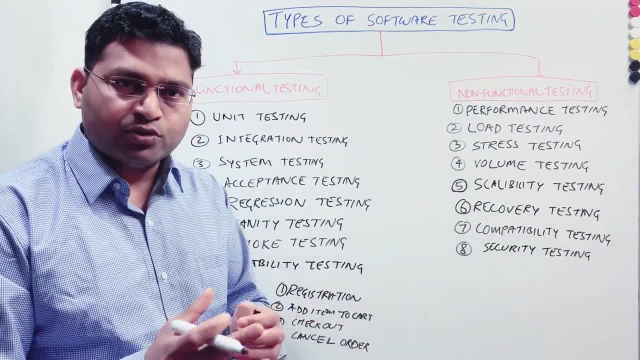 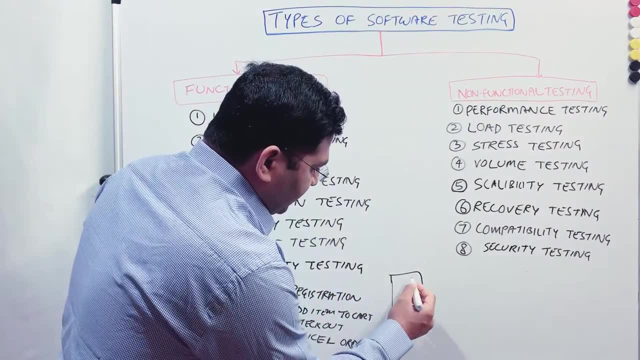 registration. So when we talk about registration, we talk about the non-functional aspect. So, in terms of registration, you will launch the e-commerce portal and you will click on the register button right. So say, for example, you have the e-commerce webpage and here you will have. 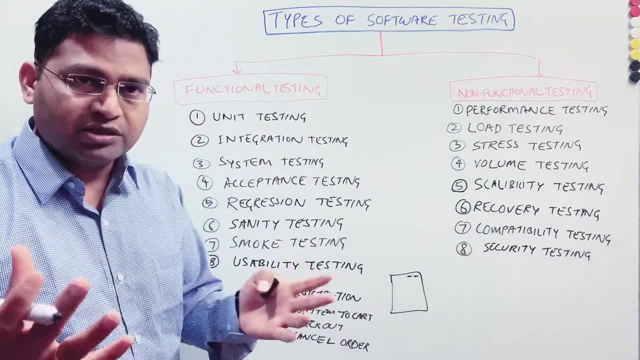 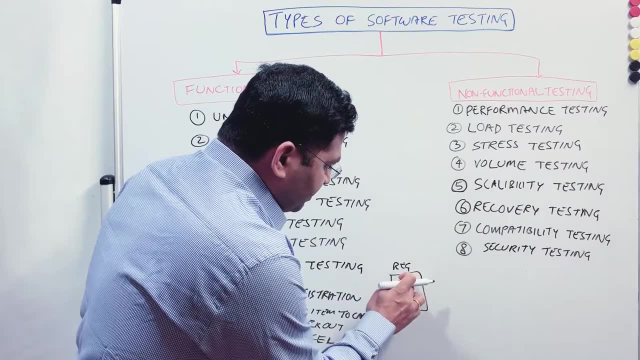 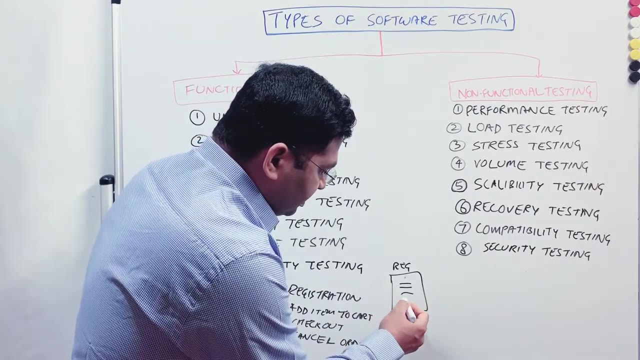 a link for the login and registration. That's how usually you see the e-commerce website. You will click on the registration link and it will open the registration page right Now. on the registration page you will have the name. you know you can first name, last name, email and then other. 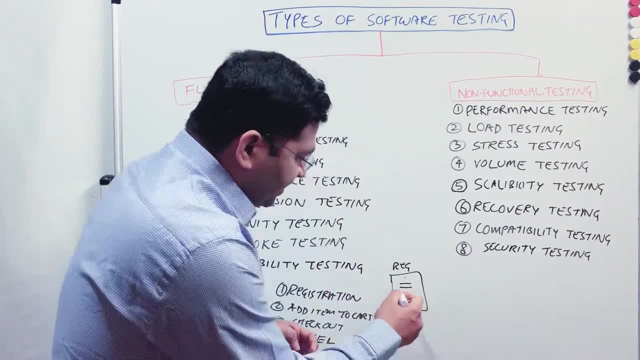 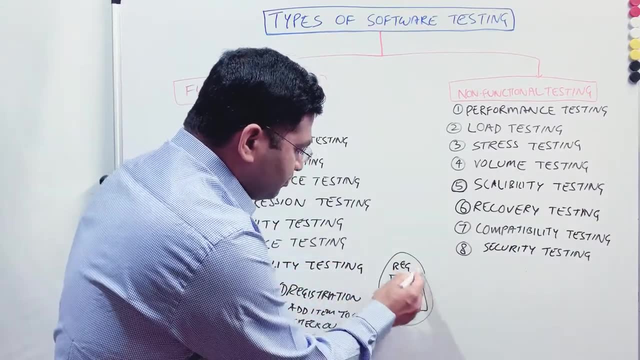 names right, And then you will click on register button and it should register you successfully. So this is the functional testing that you will do, right? So this is the functional testing, So opening the browser and then providing all the details and clicking on the register button. 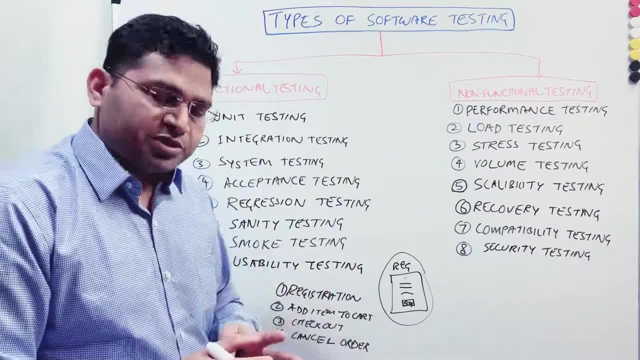 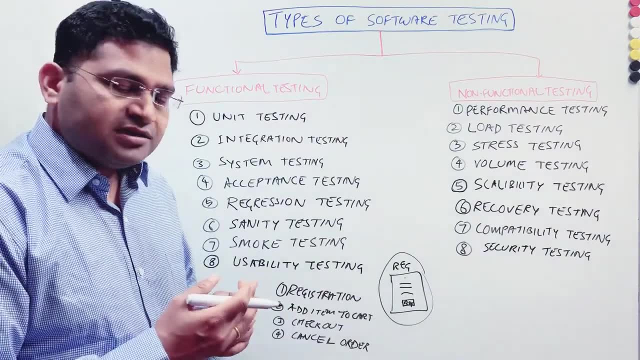 will register you in the e-commerce website. okay, Now, when we talk about non-functional aspect of this registration- say, for example, I'm trying to register and once I provide all the details and click on the register button, I will register you in the e-commerce website. 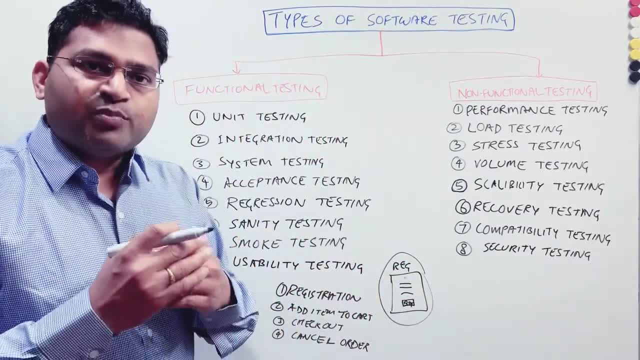 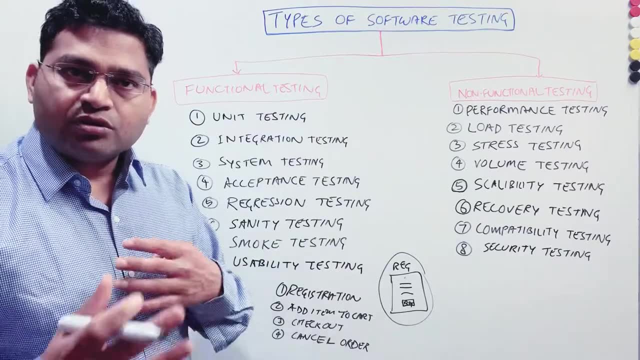 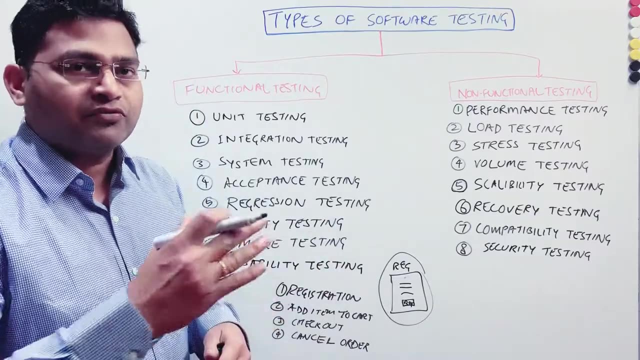 So when I click on registration, a register button, if the response or the registration takes 30 seconds to register and redirect me to the dashboard, that's not a good response, right? So because when I provide all the details and click on register button, it is taking a lot of time. 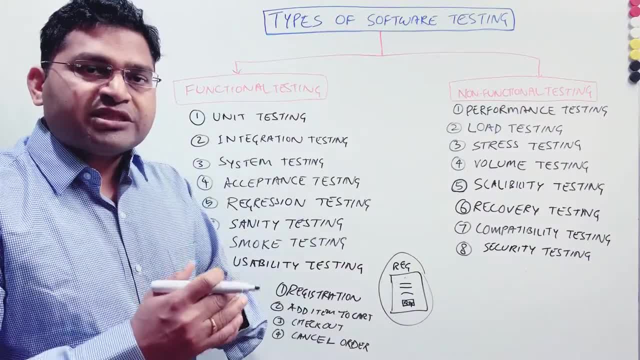 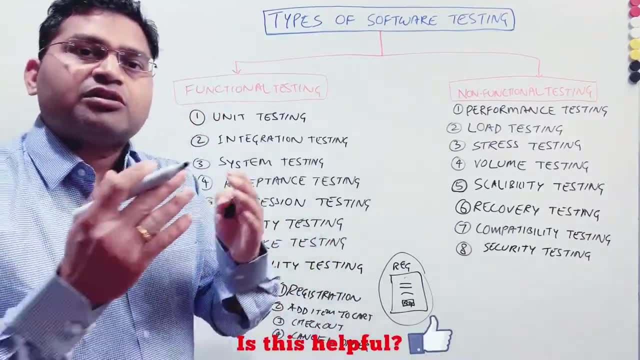 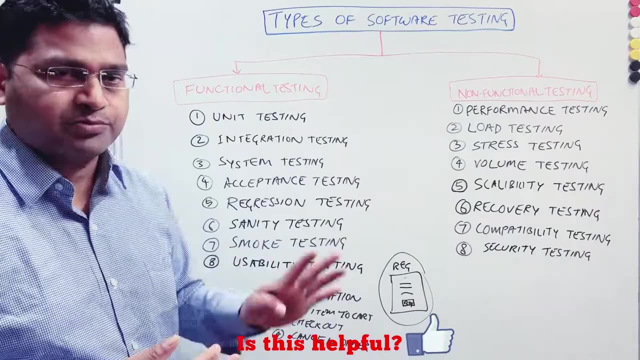 Now, when you are testing that aspect, or basically the time aspect, or how the website is performing when a user registers, that testing is the non-functional testing, right When you are testing the response time. and there are many types of non-functional testing which we will discuss briefly in this particular tutorial. So this is the case with the registration. 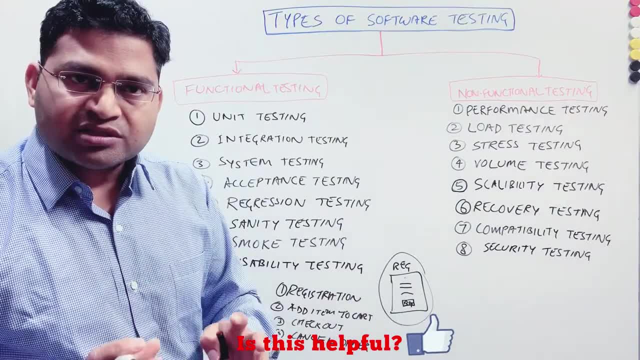 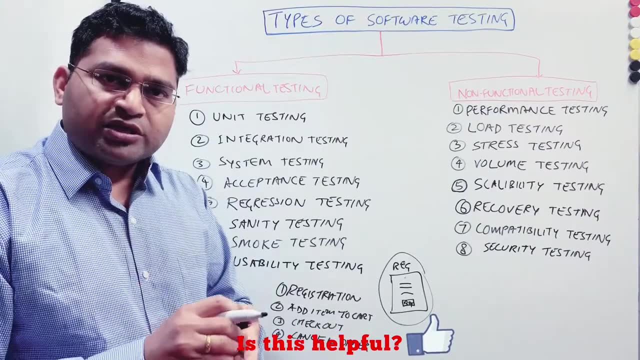 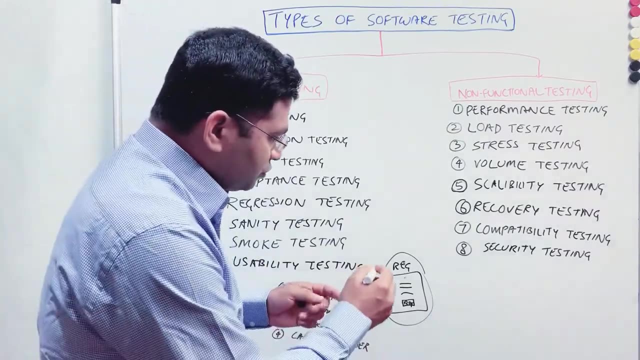 So when you are actually registering and just verifying that registration is successful, without worrying about how much time or the response time it took when the user clicked on register button and he actually got redirected to the you know dashboard page, So you are not worried about the. 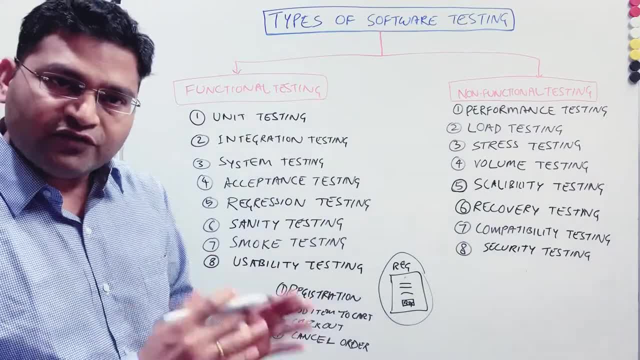 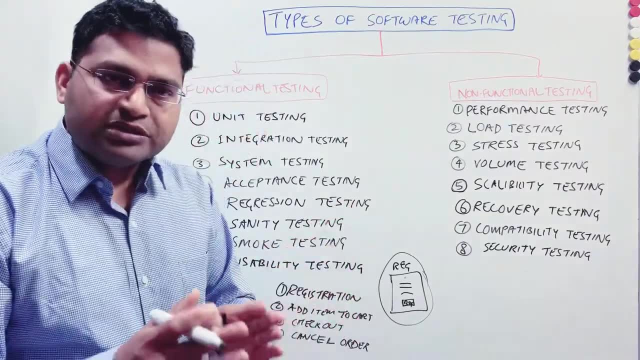 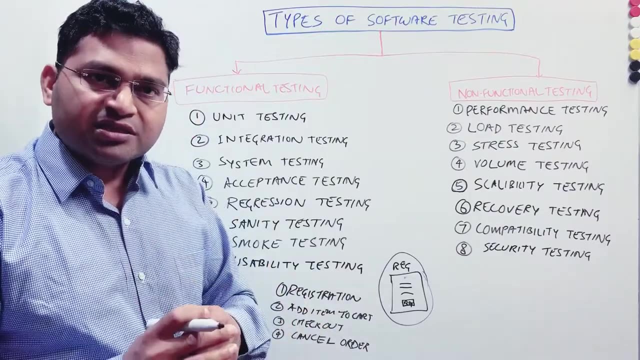 response time In the functional testing. but in the non-functional testing what you will do is you will execute this script and you will also, you will just look for the response. So once the user clicks on the register button, you will capture the response time it takes to redirect to the user, to the 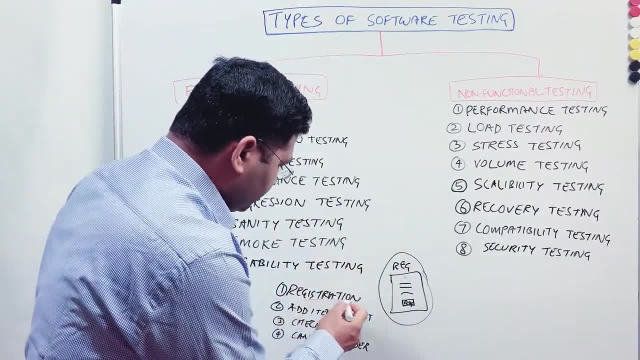 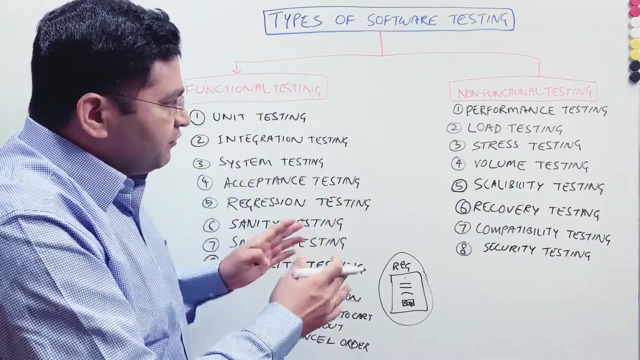 dashboard page. So that is the non-functional aspect of this particular requirement and this is the difference between the functional and non-functional testing. Now, when we say types of other types of testing, so now these are the testing types, that are the functional testing. So if I talk about the unit testing, 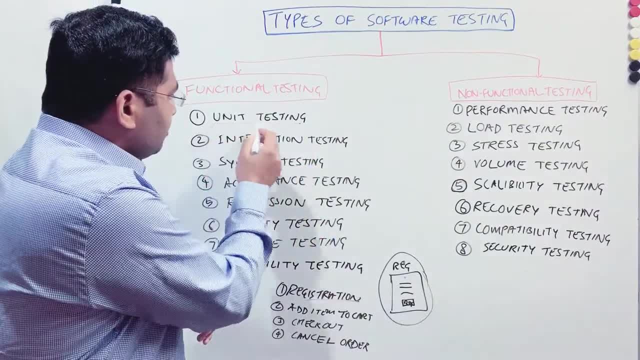 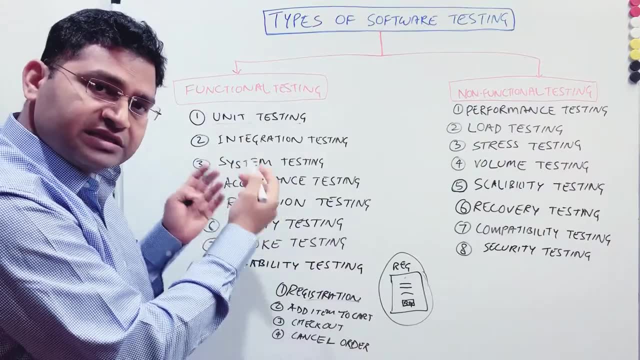 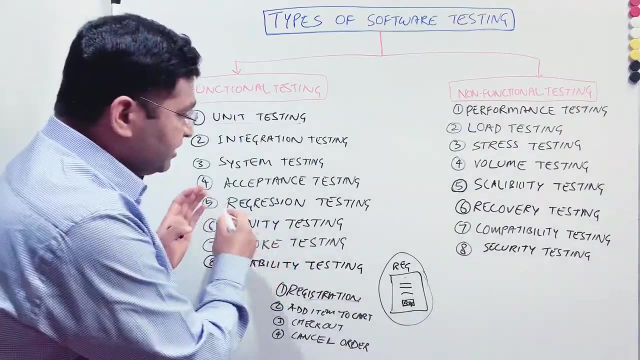 which is also one of the test levels. so that is also a type of testing, right? Unit integration system and acceptance testing. these are all test levels, along with the testing types as well. right, So you can categorize these as testing types as well. Then you would have heard a lot about the regression testing. 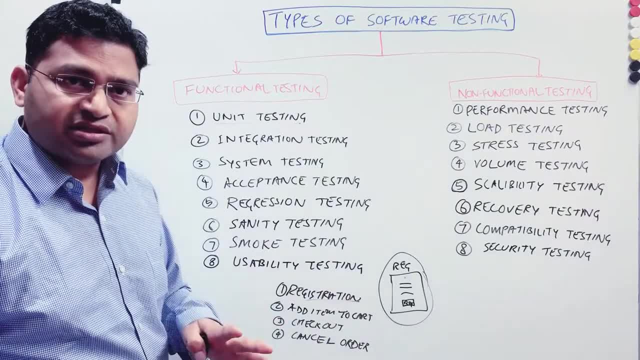 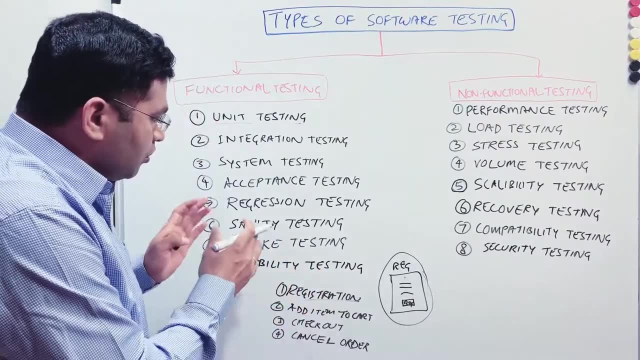 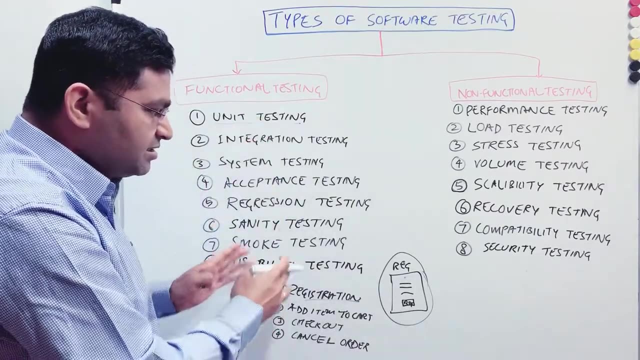 So I'll cover this in a complete, separate tutorial: what exactly regression testing is and how you need to do regression testing, Then sanity testing, smoke testing or usability testing. So all these testing types in the left-hand side below functional testing column are the functional testing That is. what does it mean That these 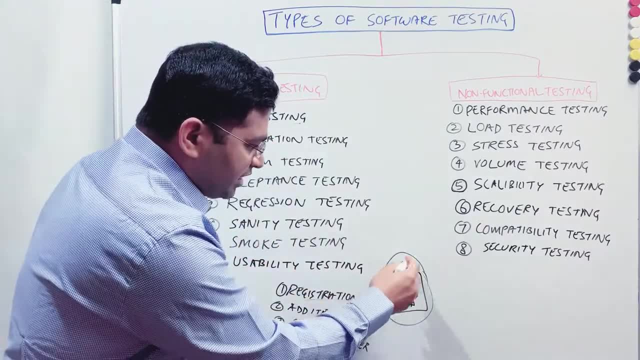 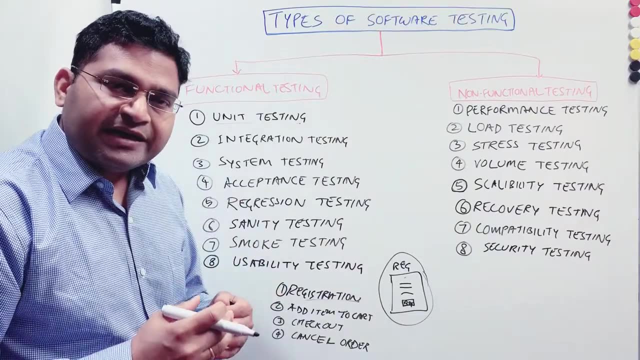 type of testing will verify the functional aspect. as we have understood, in this registration case, A tester will launch a particular application, he'll follow certain steps and he'll verify that the functionality is working fine right. So, for example, if I take an app, example, 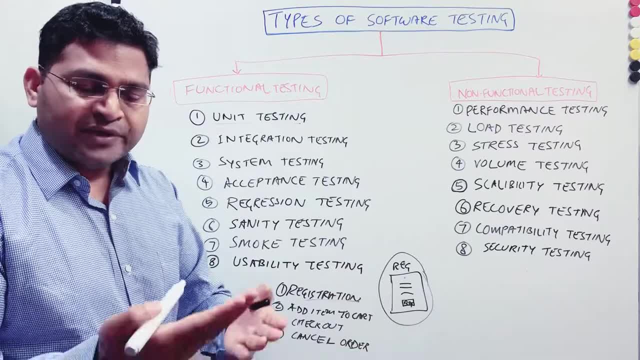 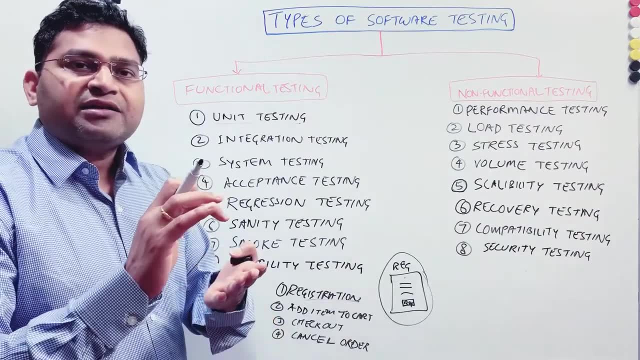 WhatsApp, say, for example. the functionality of the WhatsApp is, if I want to change my profile picture, I should click on change, select the new profile pic and then save it. right, I should be able to save a new profile pic. 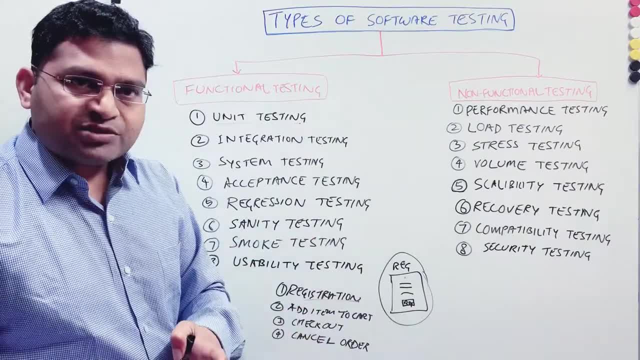 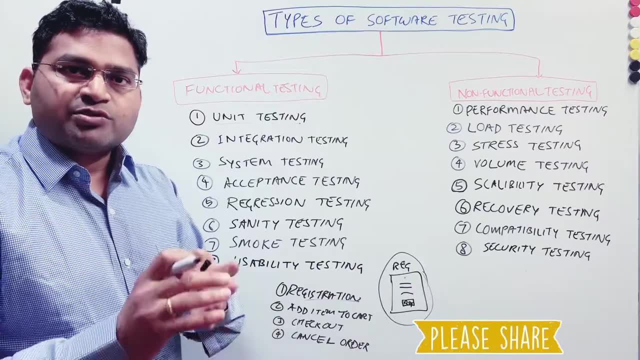 successfully. This is the functionality. Non-functional aspect of the same is: if I click on, if I select the new profile pic and click on save, it should respond. you know, within. you know, say, for example, within one second or. 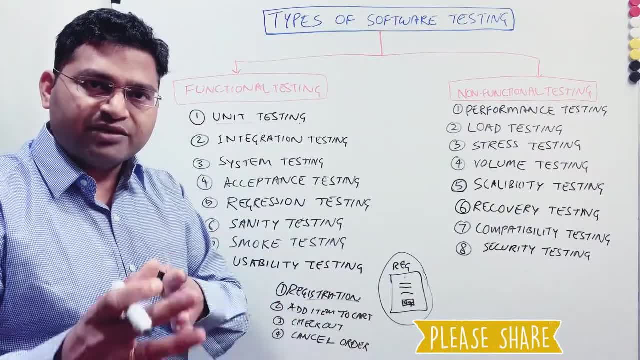 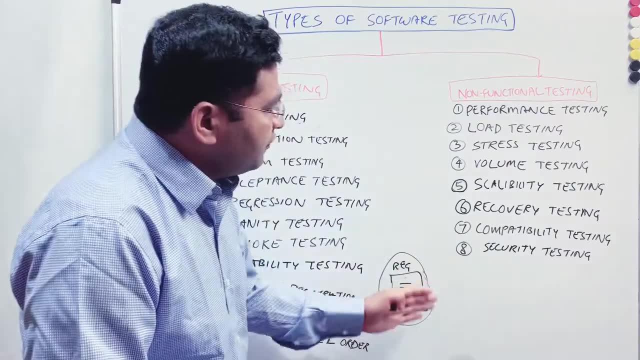 within two seconds. So that's the when you are checking the time frame that it takes to perform certain transaction. that is the non-functional testing. Now, when we talk about the non-functional testing, some types of testing in the non-functional testing are performance testing and below. 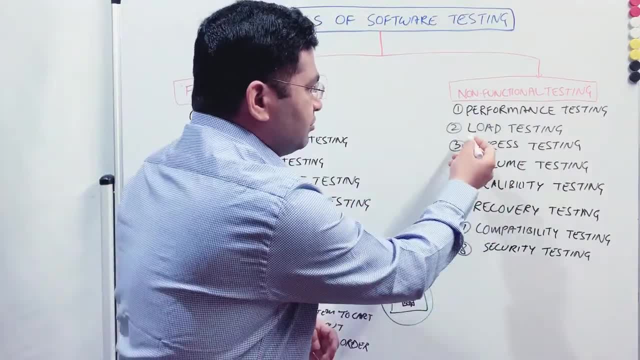 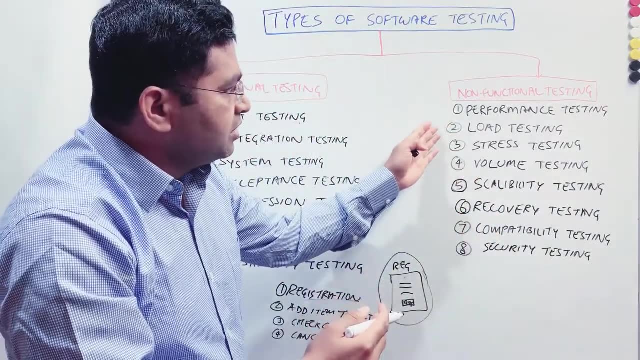 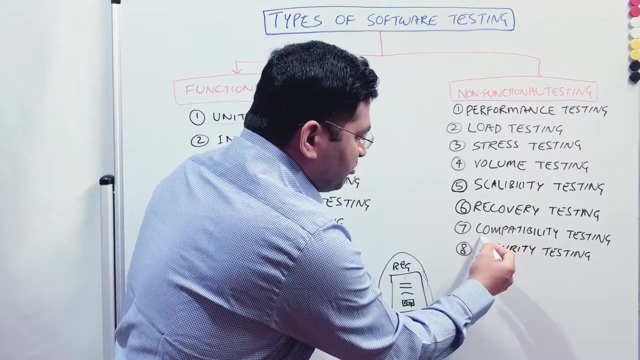 performance testing or below this performance testing umbrella. you can say you have load testing, stress, volume, scalability- all these are part of the performance testing, right? So these are different types of non-functional testing, Software testing. Then you have the recovery testing or compatibility, security testing, right So? 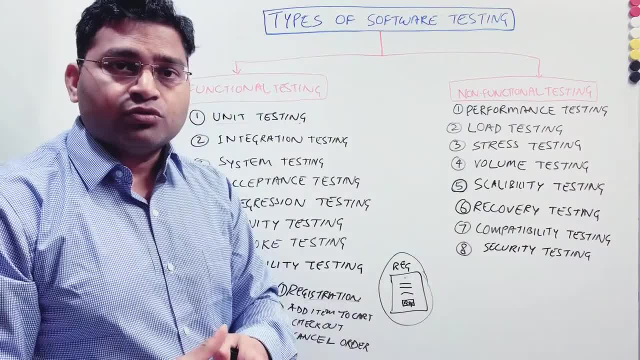 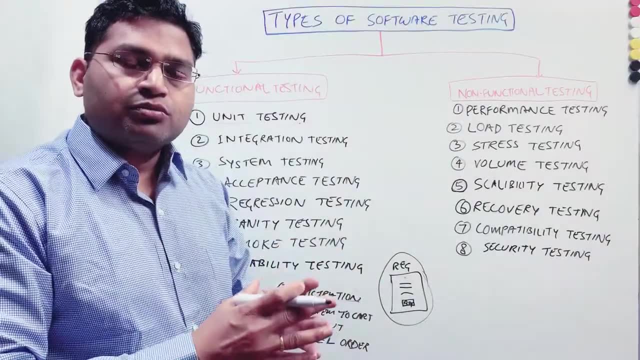 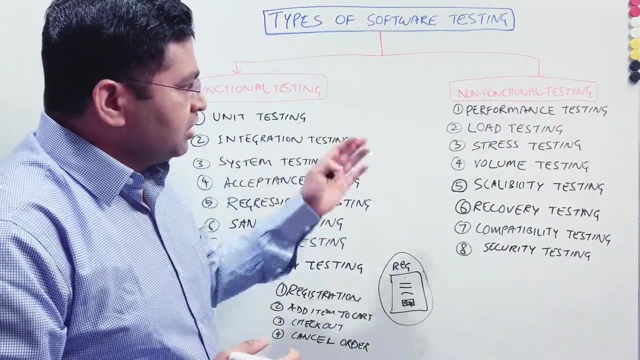 security testing is very, very important for the software. So to basically save your software from being hacked or, you know, stopping the hackers to stole the user data from the software that you are launching or the website that you are launching, right? So these are some of the functional and 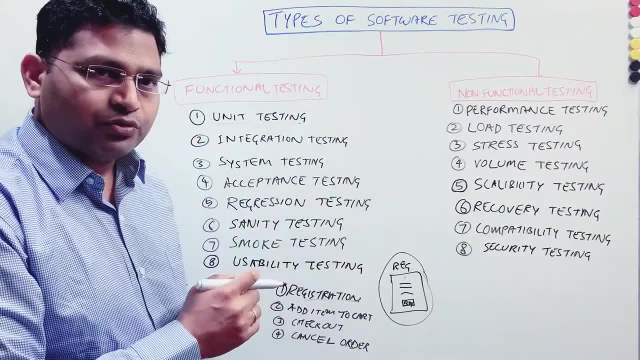 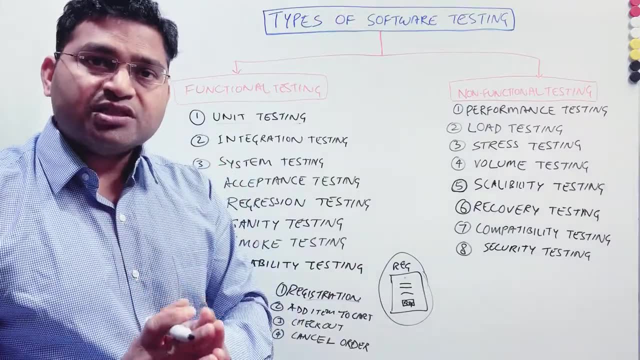 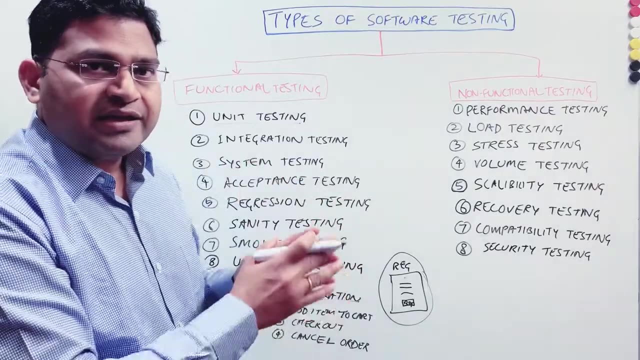 non-functional testing and types of testing that I have you know, mentioned here. If you go ahead and Google about the types of testing, you will get a lot more types of testing that you can categorize within the functional and non-functional testing, And then you will. 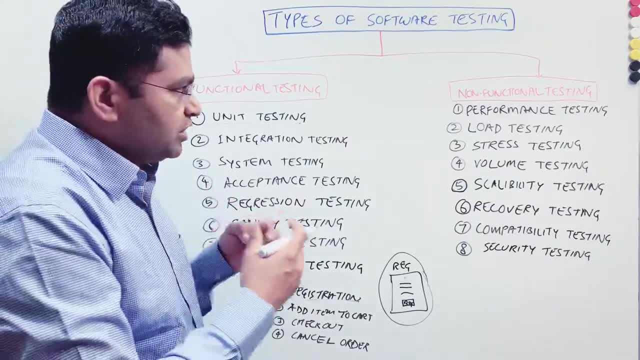 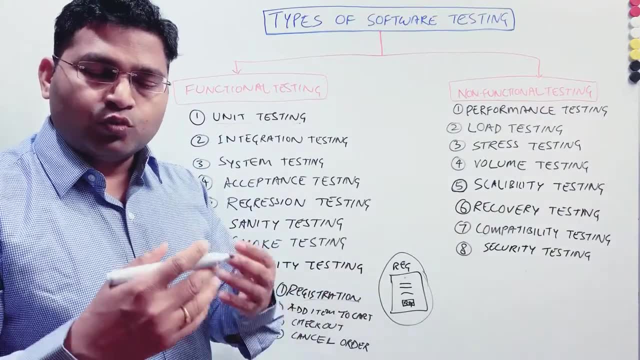 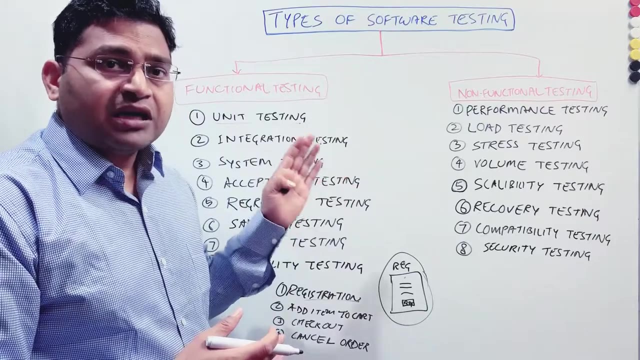 have the complete list of the testing which will help you to understand what all types of testing are there and what exactly they. you know what exactly you do within those type of testing Types of testing I'll be covering So, for example, you know I've already covered unit. 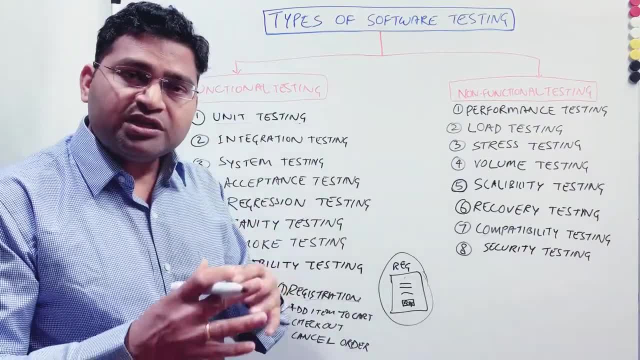 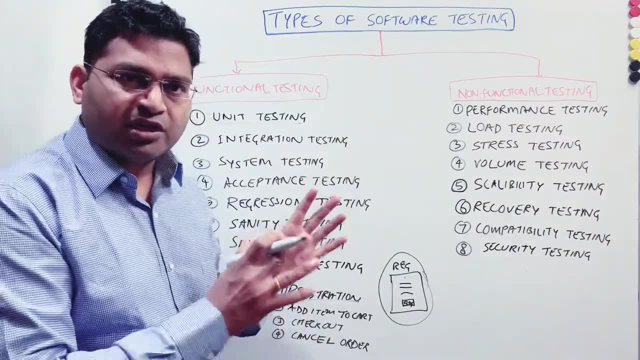 integration system acceptance. I'll be covering the very commonly types of testing that are used in the actual projects. So don't worry about them a lot because most of it will be covered. But in terms of you know, like interview aspect, you might be asked some you know. 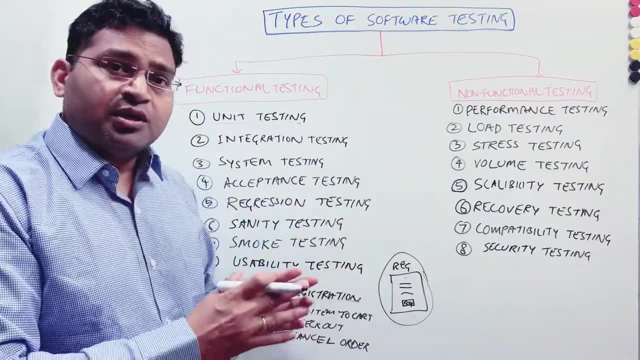 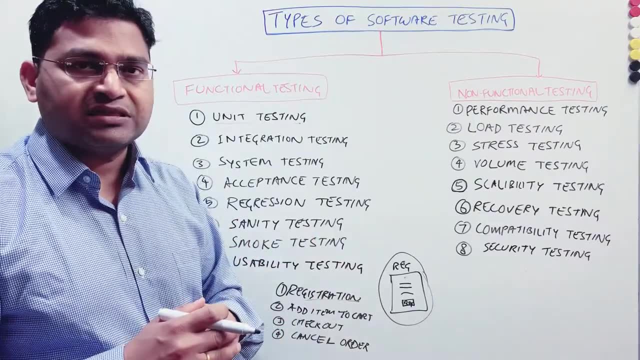 type of testing which you might not have heard before. So it's better to Google all the type of testing and get a list of those testing and understand those testing. But most of the time those type of testing are just required for the interview. They are not. 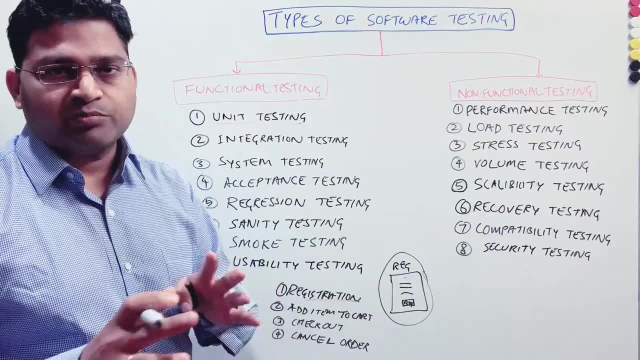 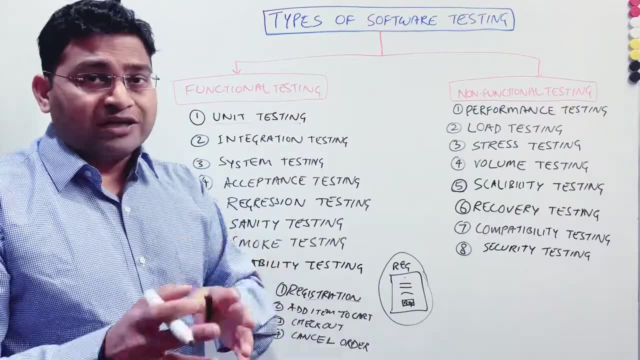 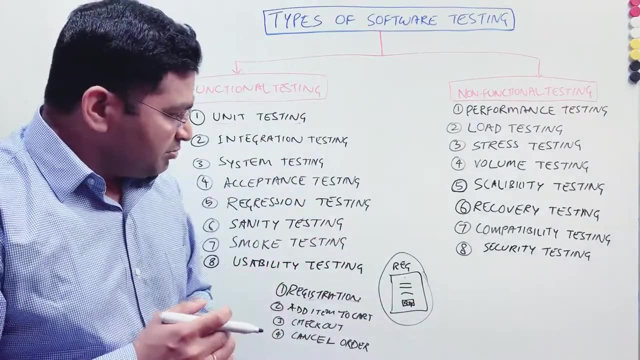 very commonly spoken or used into the software testing projects, right? So whatever is required for a software testing project or being very, you know, widely used in terms of testing types, I'll be covering as part of this series. So that's pretty much all about the types of software.